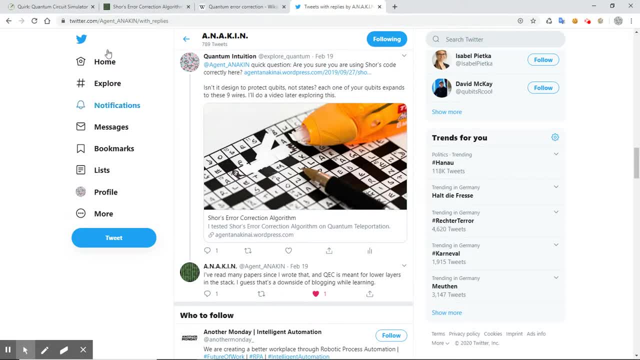 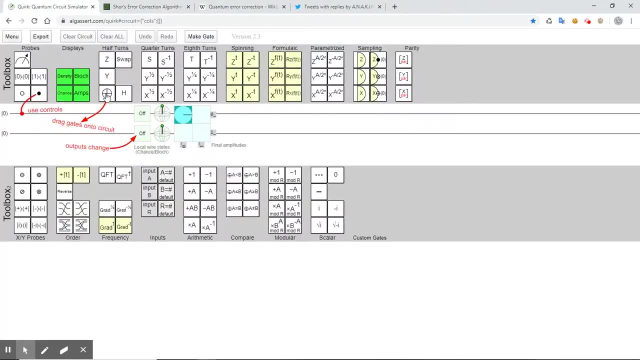 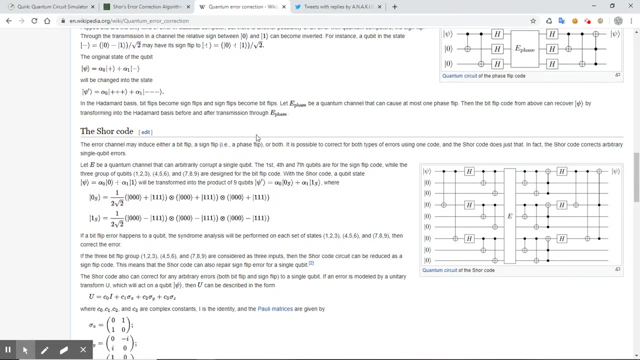 Cool. So this is a. this should be a short thing. It's just a couple of things came kind of together that I thought would be interesting to do a quick video on this. So it's about primary correction and it's not going to be here some sort of like theoretical whatever. It just kind of realized. I realized I found I found a short code which I haven't. I didn't know about before. I knew about the idea of encoding it in sort of entangled states and then using the party. 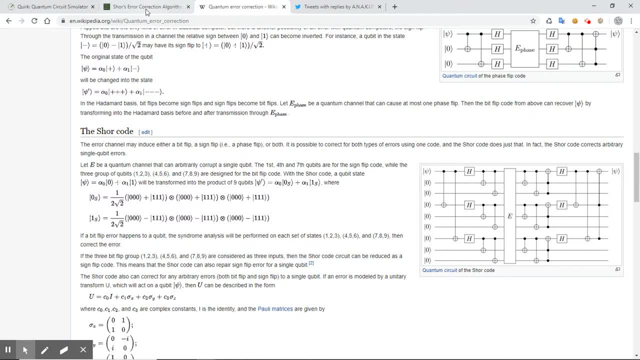 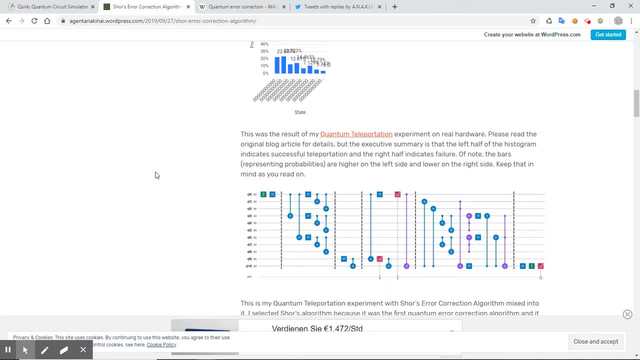 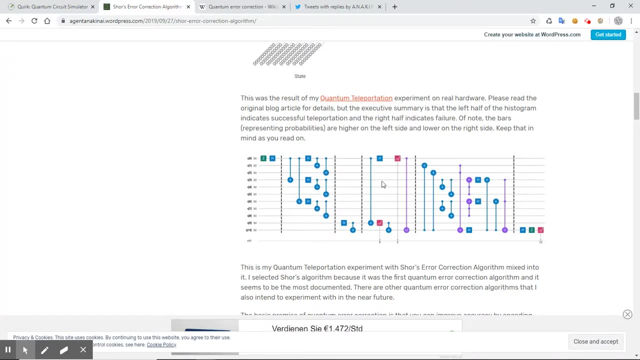 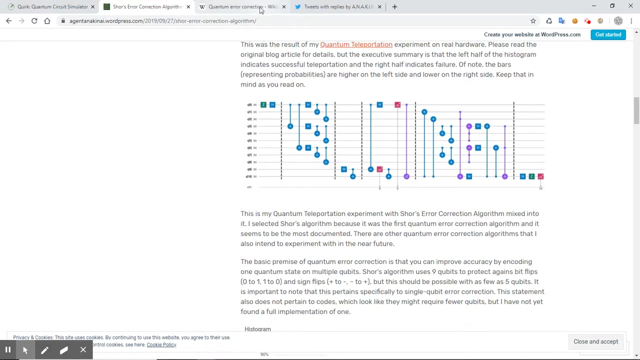 Right, I think something like that, Right. But then, because I stumbled upon these blog posts from H and Anakin AI, which basically it's, it's, I think it's older And I think he's trying to use that code with and mix it up with quantum teleportation, But I think he's not using it the right way. But I mean, it doesn't matter, He, because I basically he said that you know, he, he, 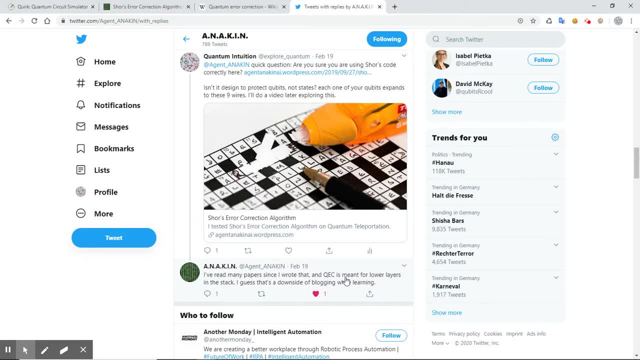 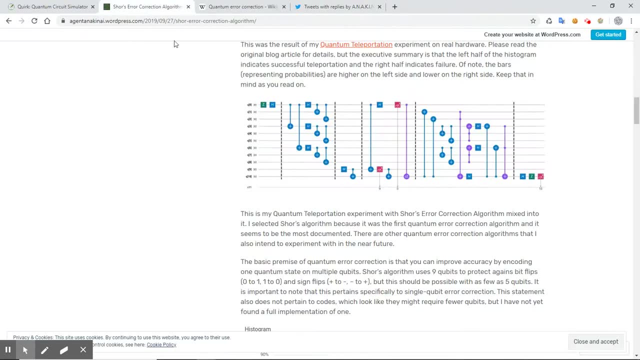 he realized that it's something that belongs to lower layers in the stack, which is what he says in his response in here. which kind of sure that makes sense, right? Because it's not something you do on a level, It's something that you do to encode logical qubits. 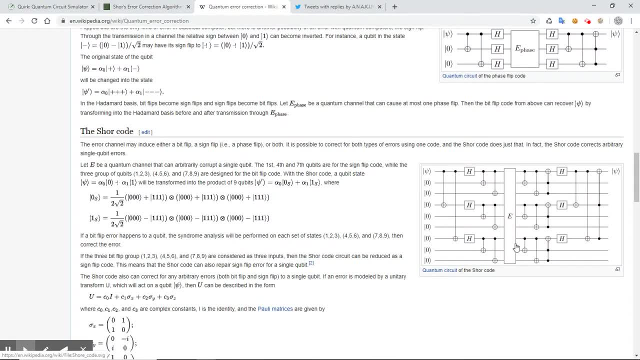 Nevertheless, I thought it would be interesting to just play with the circuit and see what the properties are of the circuit. So the idea is that this circuit in principle should help you fix both fit flips and face flip errors that might happen in this box. E right. 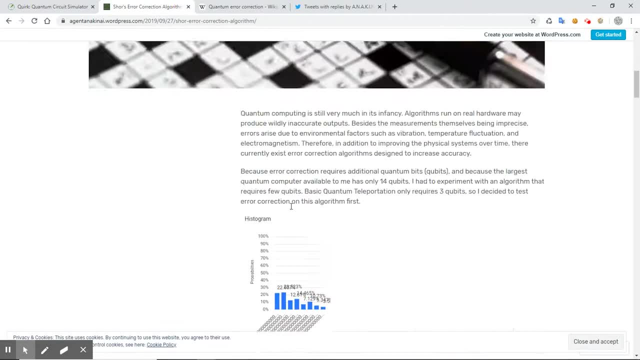 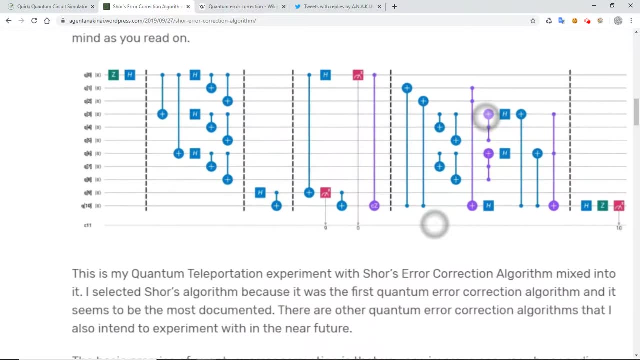 So I think the way this is used in Agent Anakin's block, it's he's trying to. I think he's trying to give me a second zoom in. I think it's trying to kind of, because this is definitely. 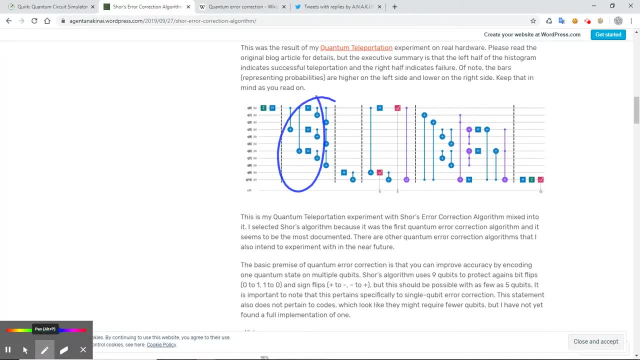 so this is definitely the error correction part And this is the same. but it's kind of flipped because I think he So he takes that state in here And then, because it's in theory teleported down here, he's basically putting all those controlled operations that. 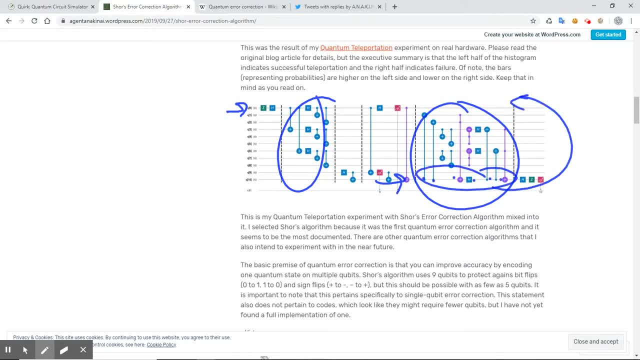 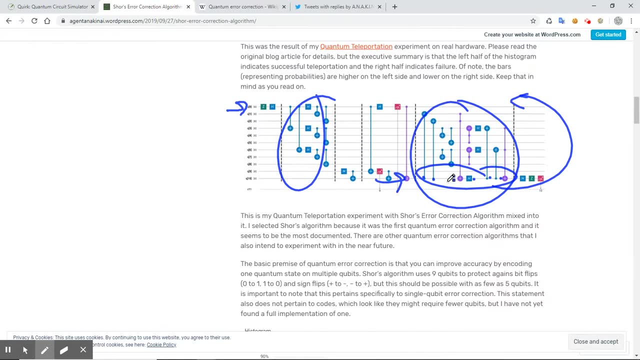 should belong to that part up here putting them down there, And it doesn't kind of work right away, And so I think the issue here is that it's not. you don't do that at the logical level. You don't do that to protect a particular state. 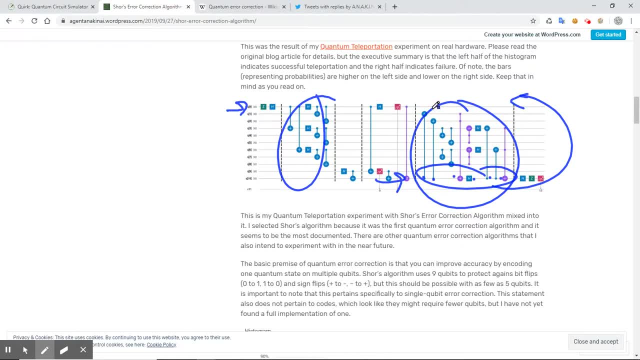 You do that per qubit, like per physical qubit, And so you represent a logical qubit with nine physical qubits, physical qubits that are entangled in such way. That's the way I. that's why I understand it. 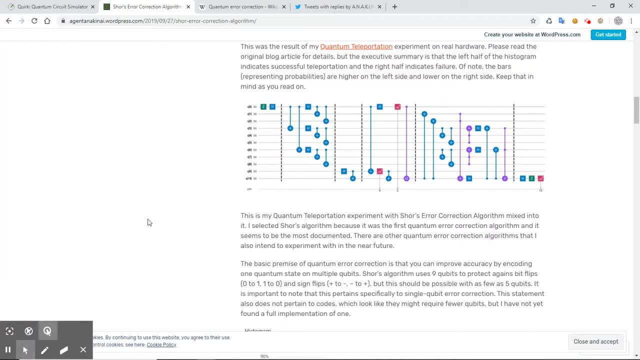 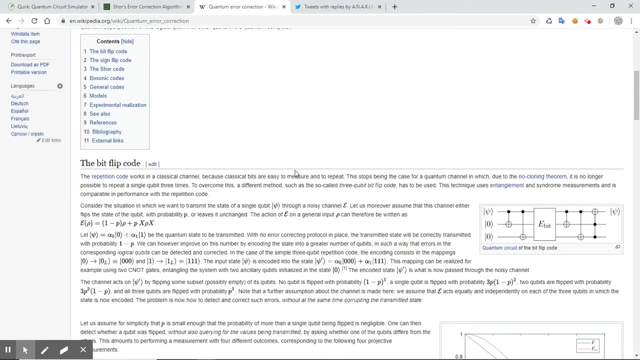 And I'm you know might be completely wrong, but that's the, that's the idea, Yeah, So that's that's the idea, basically. And so I went ahead and I found this in the Wikipedia, And so in the Wikipedia you've got these in here. 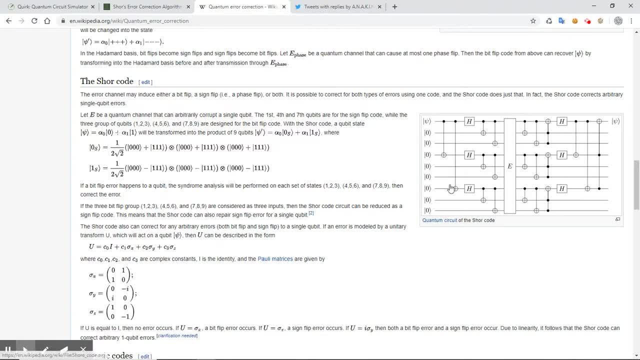 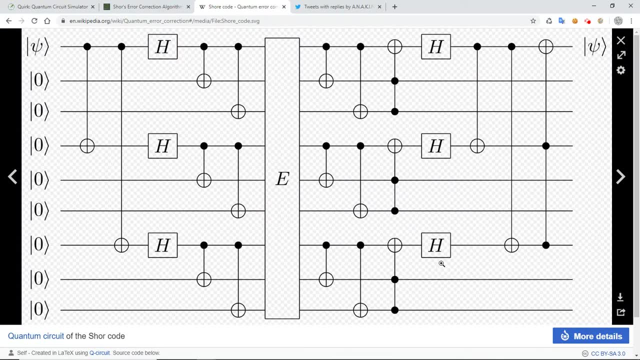 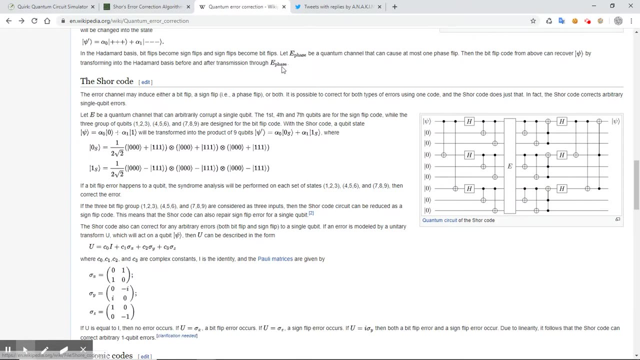 you've got like some sort of explanation, but you've got this in the Wikipedia here as well, in the shape of a circuit, And oh, cool. And so what I'll do is I'll go ahead and build that, because I think it can be interesting to. 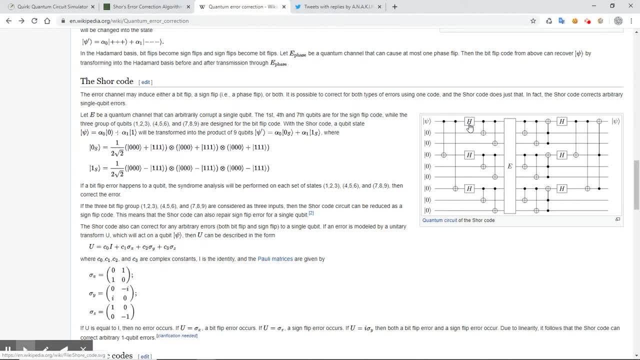 to basically analyze the behavior. I think, basically what those things are doing in here, what those blocks are doing, is the phase correction And then I think just intuitively, and then these plus these, or in particular these is is doing the sort of the flip correction. 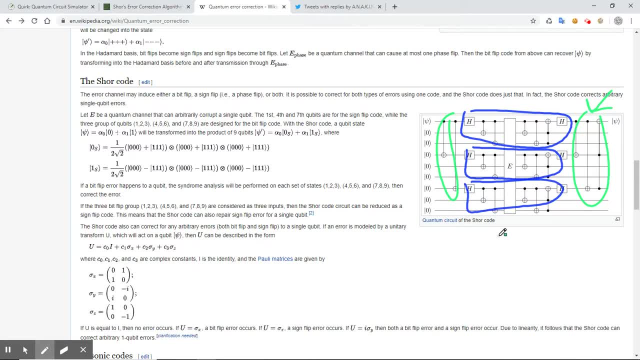 the 0-1 correction And the concept here is that it's going to basically correct based on what the majority of the three, these three registers. If you think of these three registers, you know what the majority say, then this is going to be the value that's corrected towards. 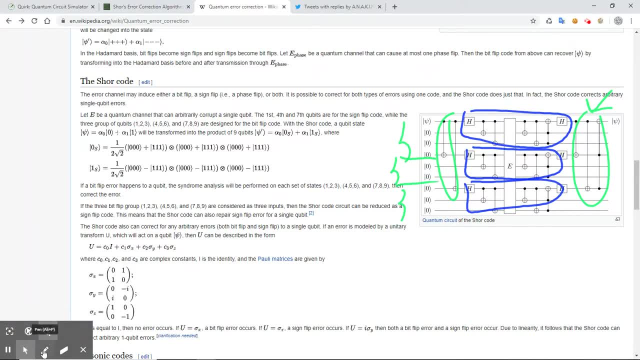 I think so, but let's give it a try and let's play with this a little bit. So I'm just going to- you know I'm not aiming here at doing anything concrete- just playing with the circuit, seeing if I kind of you know, can understand this intuitively. So let's go ahead and build this. 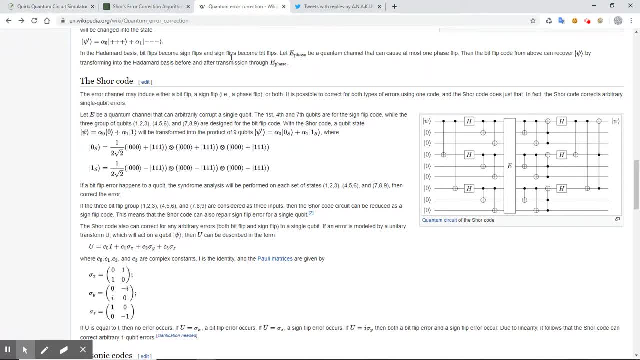 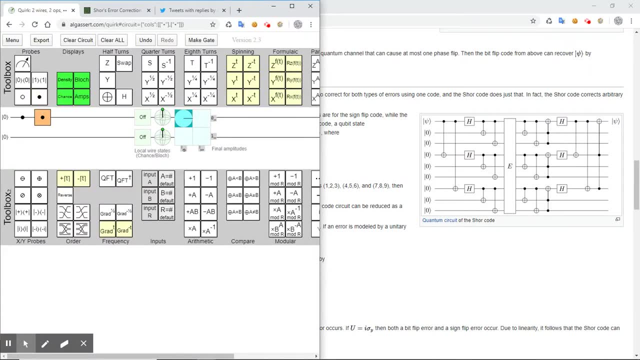 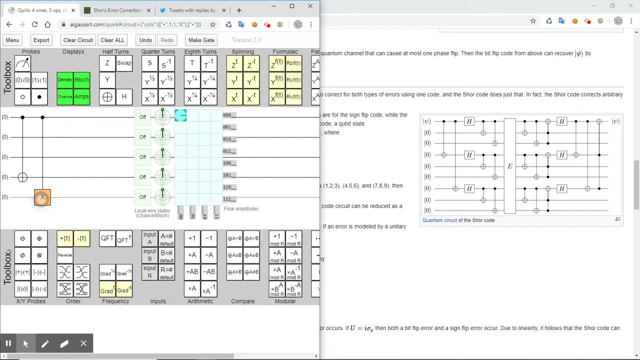 And let's see what's the best way to do that. Maybe side by side, side by side. So we've got two control beats here, then we need a, so we're going to play with these and that way. yeah, I think that's. I think that's it. 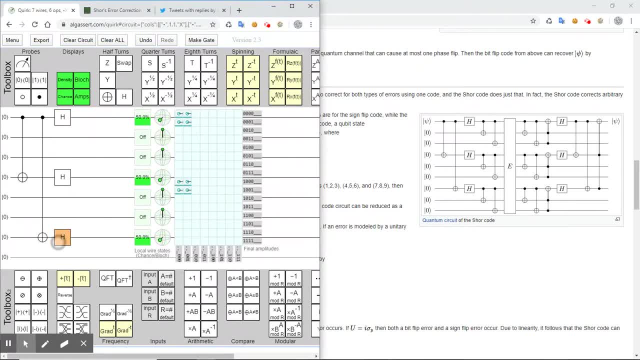 Then we've got a hotmart, we've got a hotmart, we've got another hotmart And now we're doing, now we're doing more control beats in here, And so we're doing these and these. Now we don't want, I don't want these to look like that. 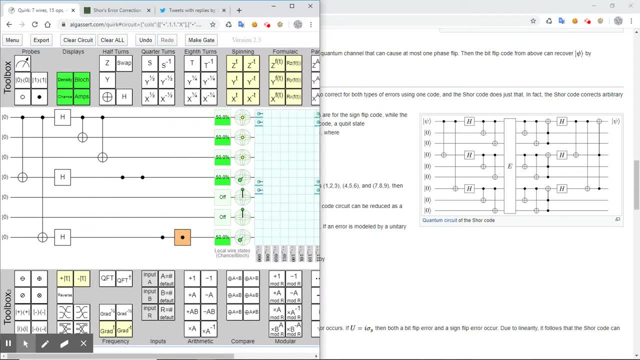 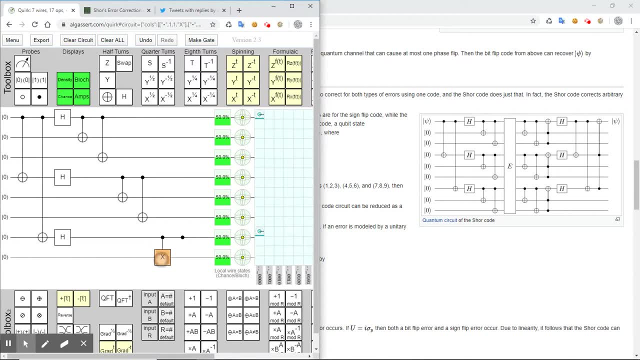 So that's definitely going to take some extra space, I think, here to make sure those things don't get connected where they should be. So that's definitely going to take some extra space, I think, here to make sure those things don't get connected where they should be. 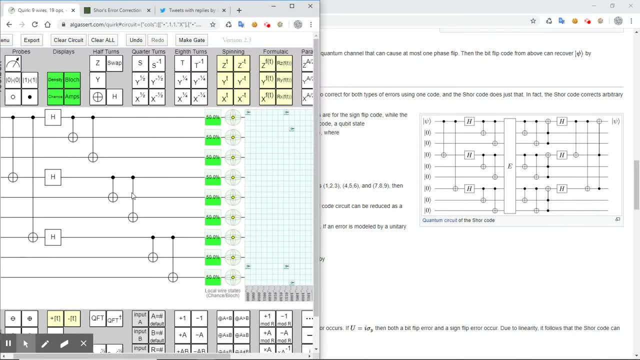 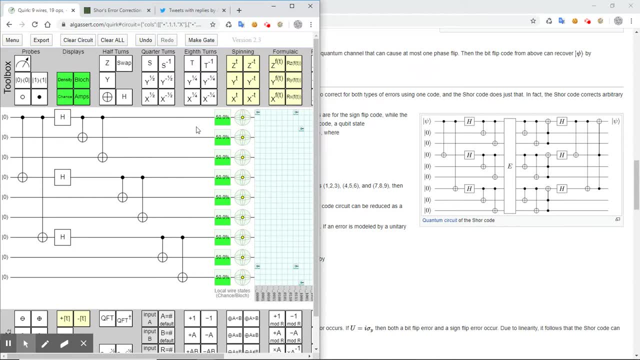 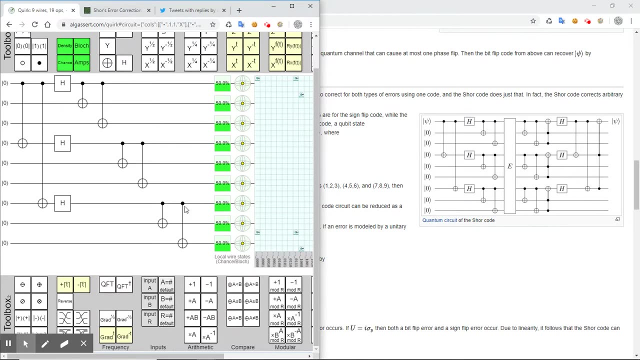 Exactly, And now, basically, now, basically, we can apply in here the, the, you know whatever error we want to simulate that that's happening. So I'm gonna, I'm gonna add maybe a bunch of these gates, just to work. 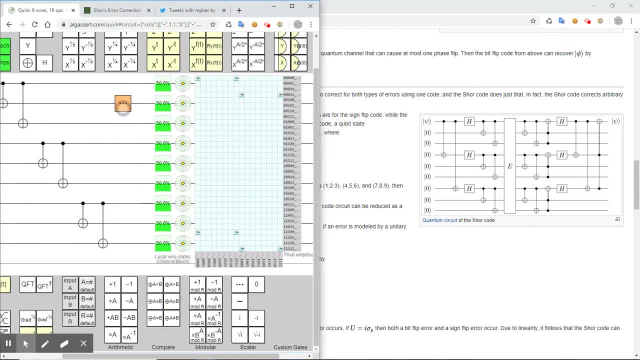 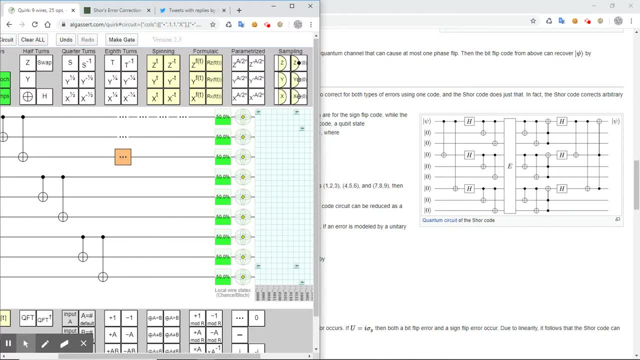 So I'm gonna, I'm gonna add maybe a bunch of these gates just to work. So I'm gonna, I'm gonna add maybe a bunch of these gates just to work, to just to mark it, just so i know where this goes. so i'll just do something like this. so this is. 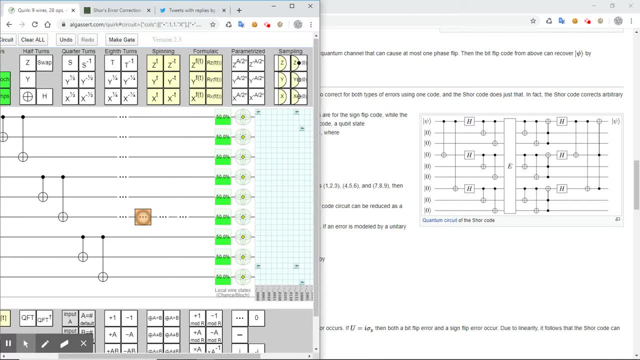 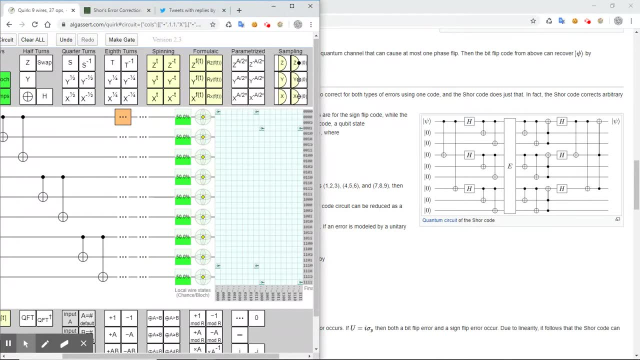 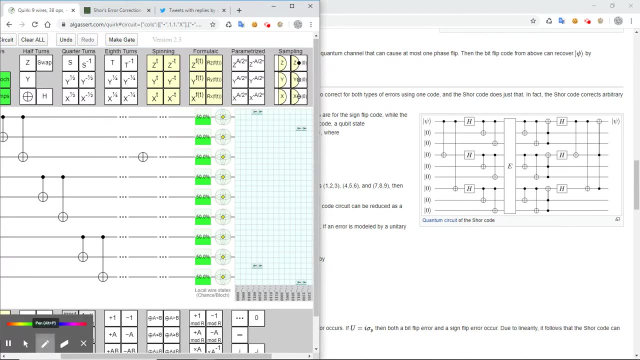 where. so this is where you know where this whole thing is supposed to be. can i just- yeah, i think i can copy that, so i'll just put it in the middle, right? for example, we'll say: i don't know what happens if we've got a bit flip in here, right? so this, this would be simulating an air, a bit flip. 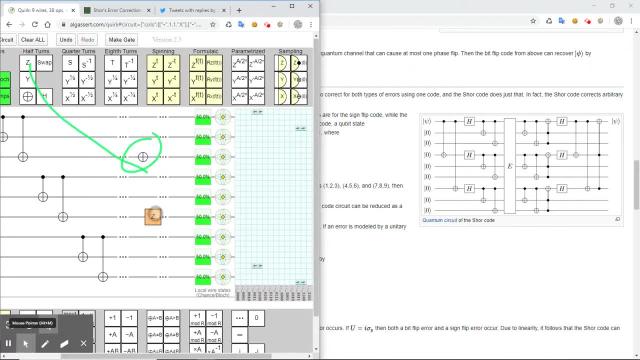 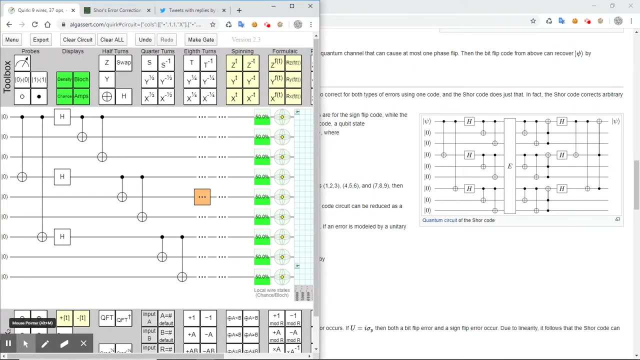 error, or what if i got like a whole a uh z flip, like a phase flip here, right? so that's, that's the way that we're gonna approach these. um, let me get rid of this one now. so next is basically uh and doing or not, undoing that, but so these and these. 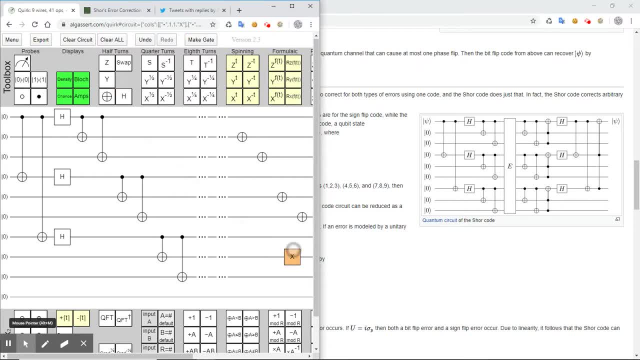 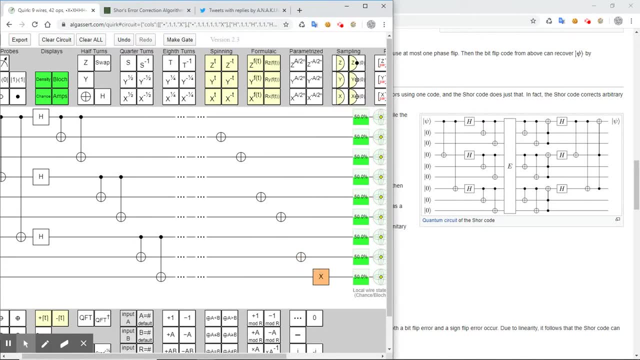 against these and these and these, okay. so at this point i think i just need to make that a little bit bigger. and now we're gonna get the controls in here and connect it. connected in here, so this just goes like that, and then these guys go down here. 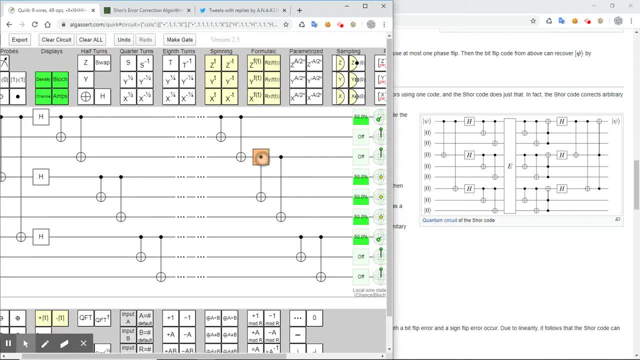 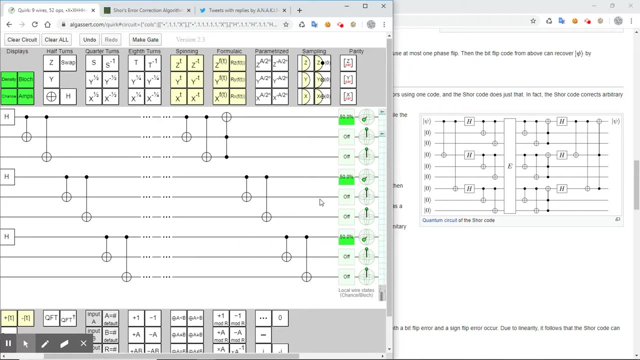 and then we've got basically a sorry, those go like this, and then we've basically got that kind of that kind of notion, okay, which is probably going to do the correction. that's the part that's correcting, so that definitely takes some extra space. what is this? sticky keys? 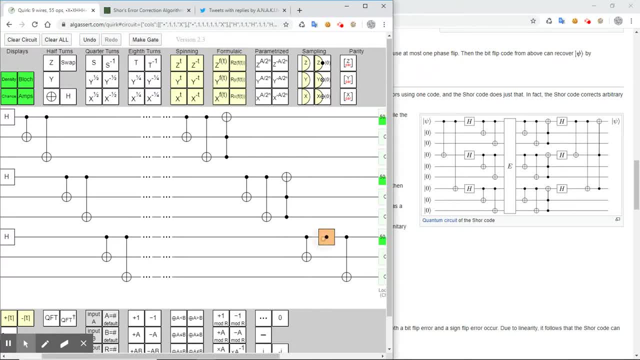 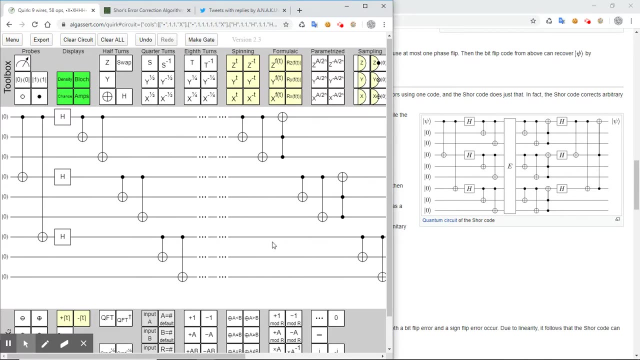 i don't want sticky keys. what are you doing? um? so i've got this one. finally, here i. there's no way, i think, i can put those darkly below each other, because they're just going to connect. so so i gotta, i gotta, have it this way. 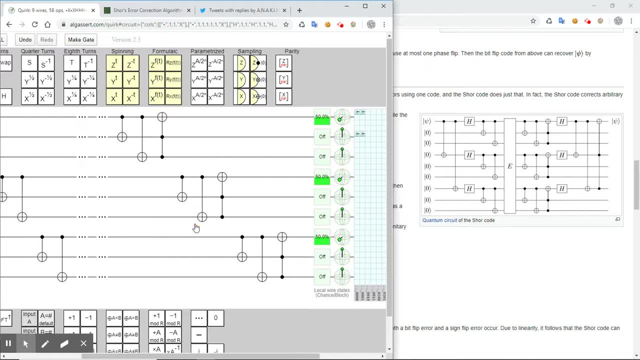 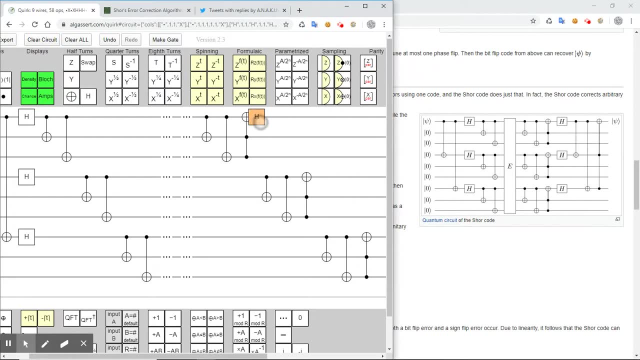 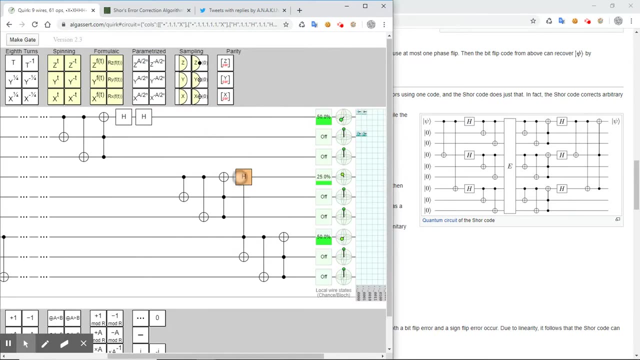 sadly, which just makes the circuit a bit bigger than than i'd like to. um, then we've got a hotmart in here, and then we've got another hotmart in here, and then we've got another hard mart in here, and then we've got on the higher mark in here and at the end, basically we need 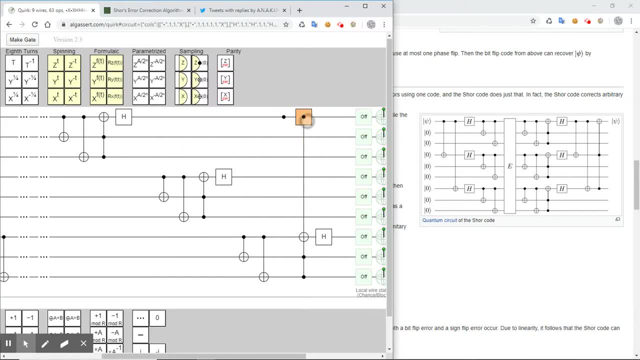 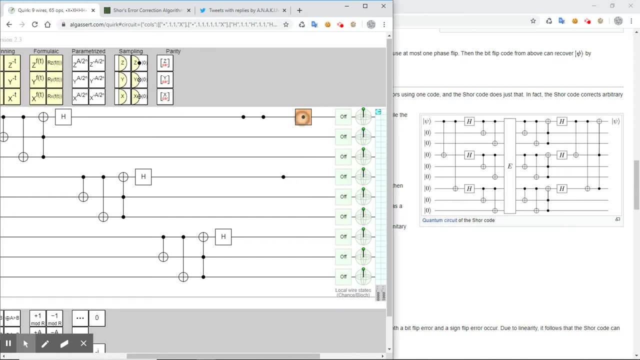 a, we need some, some stuff in here. okay, so we need those other control knots. stop on these sticky keys. and then we're going to do the same thing in the other side, and then we're going to do the same thing in the other side, here and here. 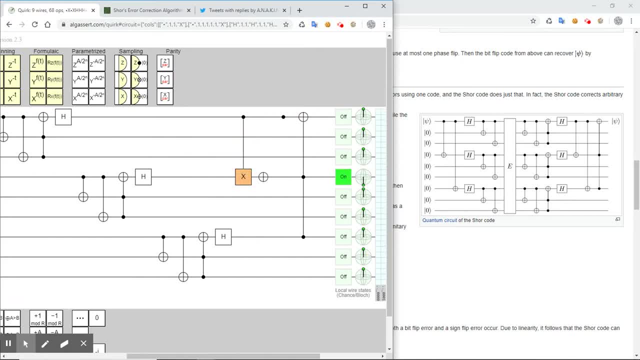 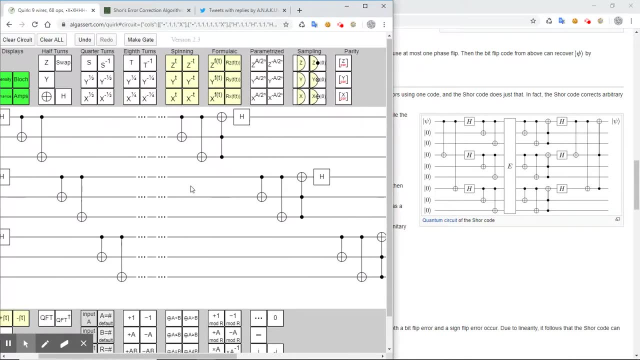 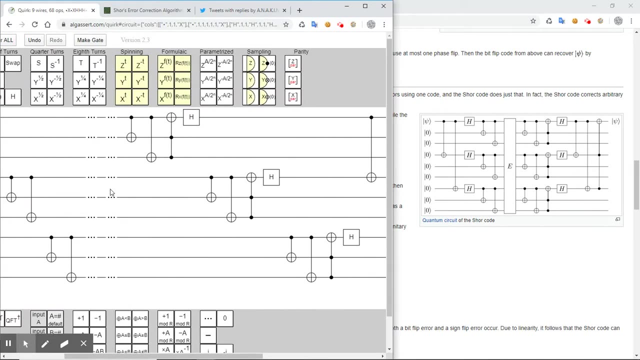 basically, i i have, i have the impression i know where this is going, but let's see, i think i got it right now. i think i think i got it right, so this shouldn't have affected anything. it's all zeros right if i in theory, let me save that. 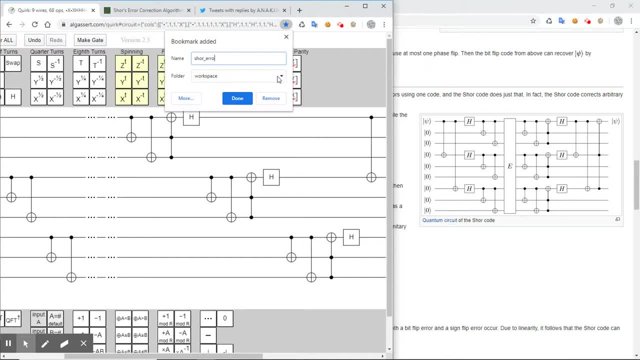 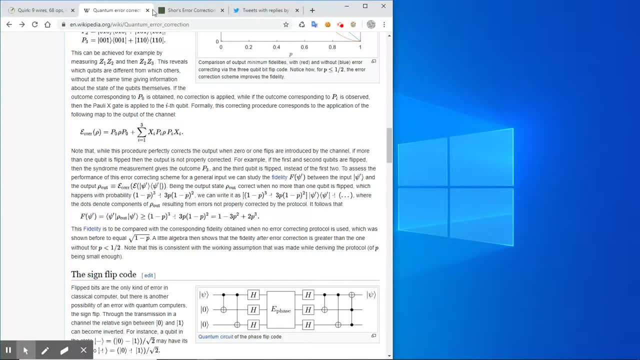 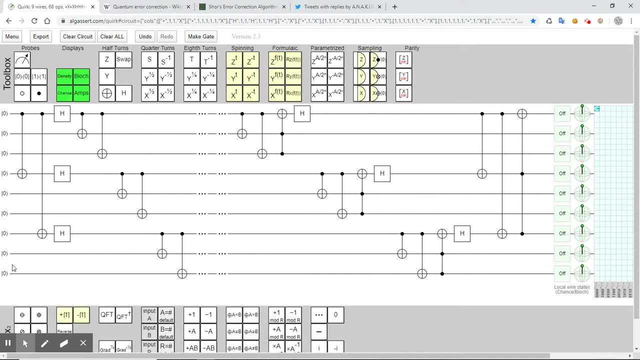 i'll bookmark that into a shore error. uh, cool in theory. let me just put that back in here. if that is a. uh you know, if i now whatever state i put in here should not in here, sorry in here. right, should kind of stay the same at the end here. so we're going to put a block sphere because this: 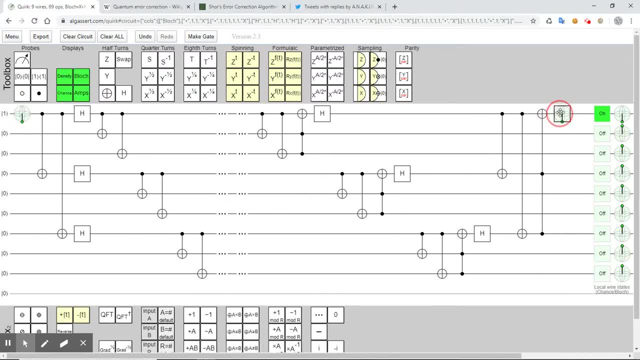 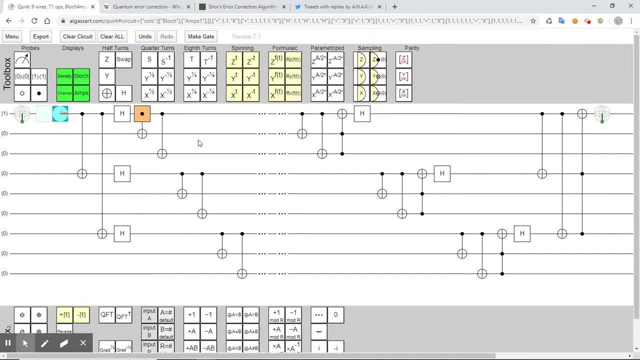 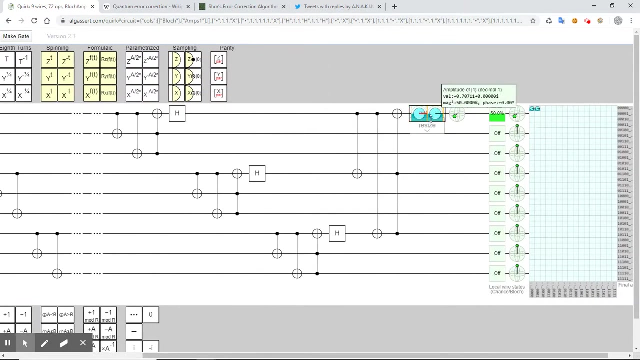 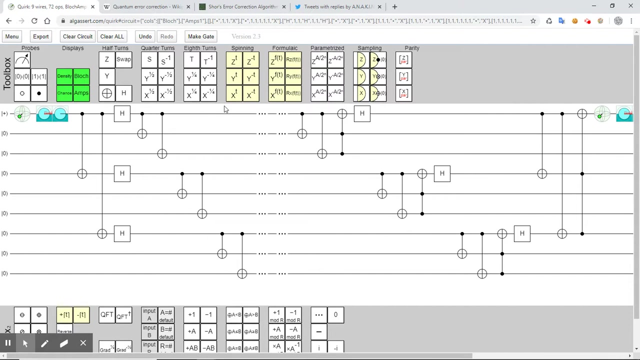 is just for um, for one qb, okay, so blocks here and also take a look at the amplitudes and just so you know, we kind of get the phases in there. so you know, if it's a plus state, then we've got this, and then it's kind of you know the same thing here right now let's play with this. so if i 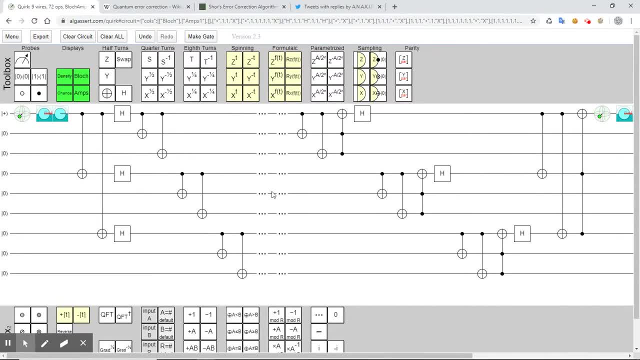 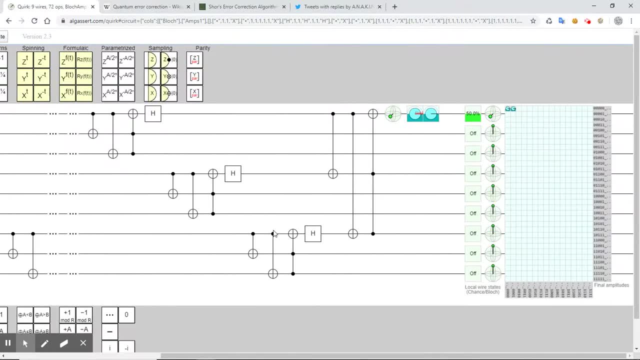 now, or maybe i'm hesitant. i would like to pack all this, but i don't want to pack it because i want to try to. i want to try to. i want to keep those control nodes and hard limits, and we're not visible, so i can, i can sort of think about what the circuit is doing. but let's play with um, let's. 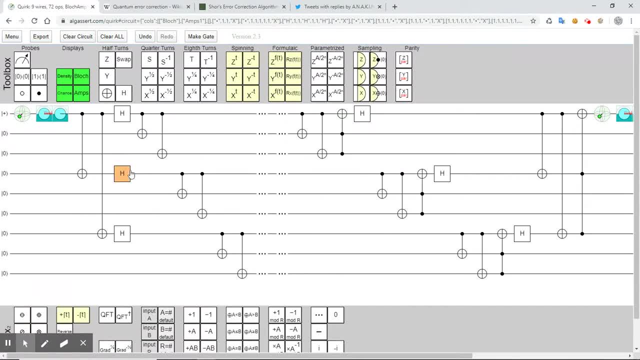 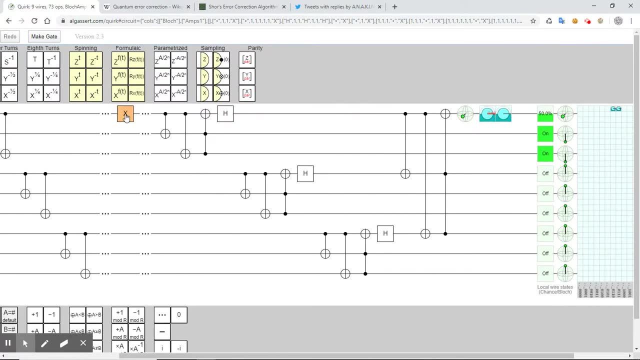 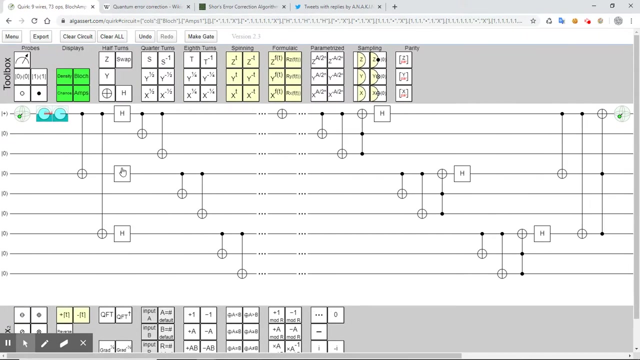 now simulate, for example: uh, a, uh, i don't know a there's an error right and this gets, there's a bit flip in here, cool an error here now, so i can just pull, so it's kind of corrected right. and again, remember this is supposed to be like. the idea here is: um, you're not supposed to, this is not supposed to, you're not. 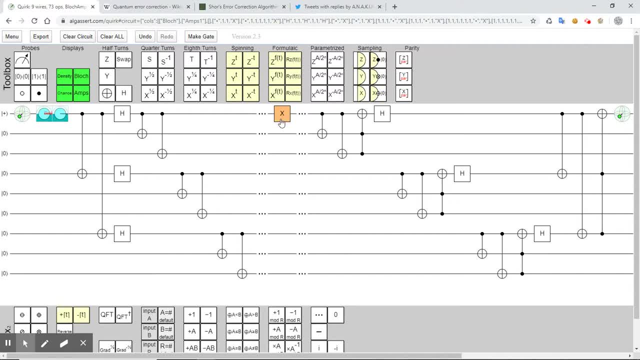 supposed to put- put a circuit now in here and do and and this is kind of supposed to, you know, shield it or something. this is just to um kind of error, correct that cubit, that wire on that we have here in the very top. um, so this is something that we should do. 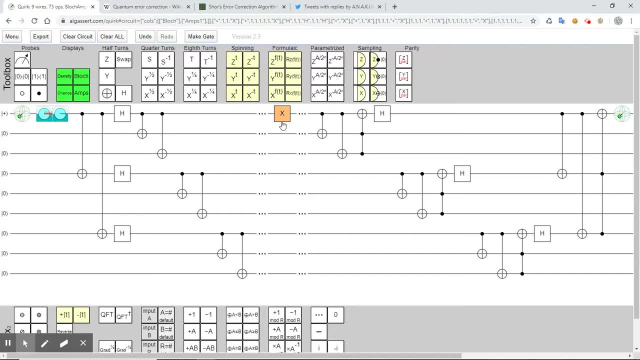 that you don't do at the circuit level, at the logical level, when you develop an algorithm. this is something goes one level, one level below in the stack, in the sense that this is something that the hardware does right. so you would treat those nine wires in here as one logical qubit. and so if you, if you would, 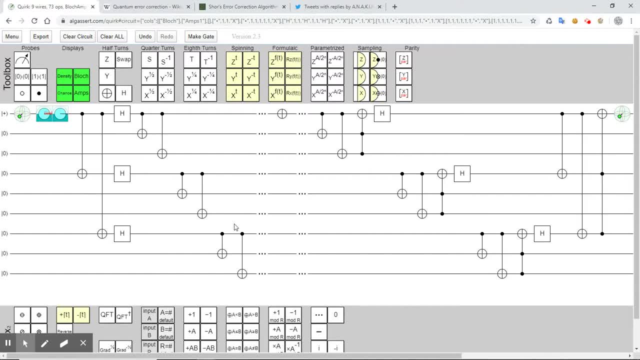 want to implement in algorithms an algorithm set, say, for example, quantum teleportation, that's one qubit for you. so you need these nine qubits two more times because quantum teleportation needs basically. quantum teleportation basically needs a- what's it called? there was a. what's it like? three qubits I. 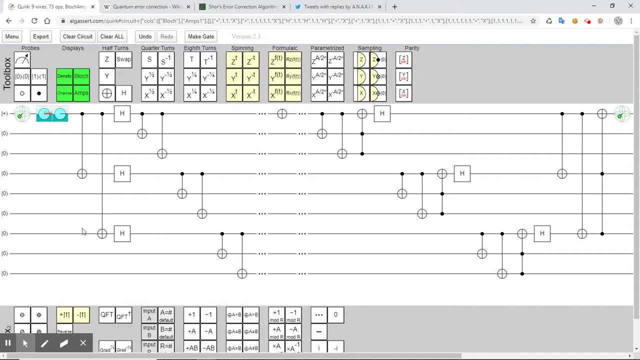 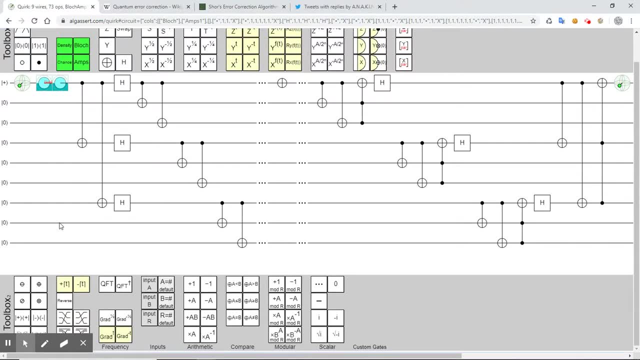 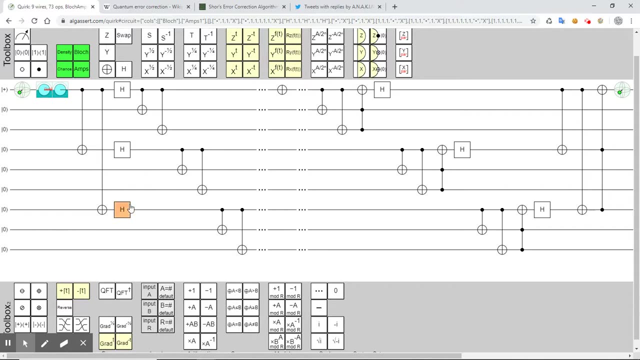 think, yeah, so, and so you could of course then kind of maybe try to simulate that. I think I could do it with quirk even. I think it supports up to 16 qubits, but that would be quite insane, and then you could. then you can think of: 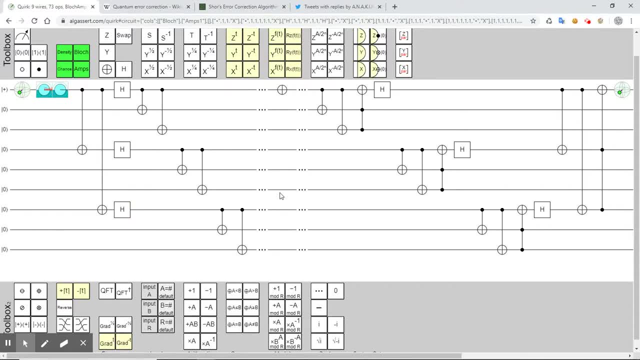 you know, you know how does an operation, how does the control not look like right, like it's not that you can't just control, not here, like you got it, you got a. it's almost like you got a control, not three like out of you you would have to this. 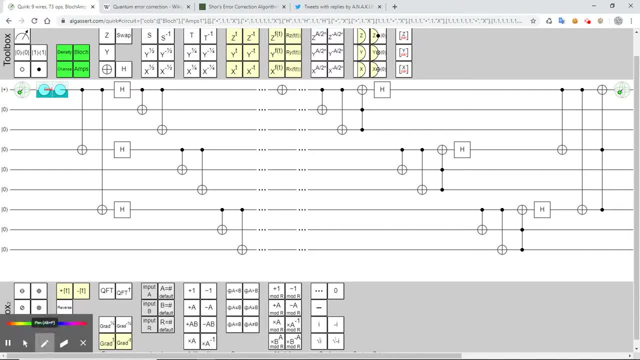 three times like one per register, because I like to kind of think about these being sorry, these being registers like this is, you know, not wrong, this being one register and this being another one? right, and so it's like, yeah, because I, inside each register, these are additional to keep. it seem to be. 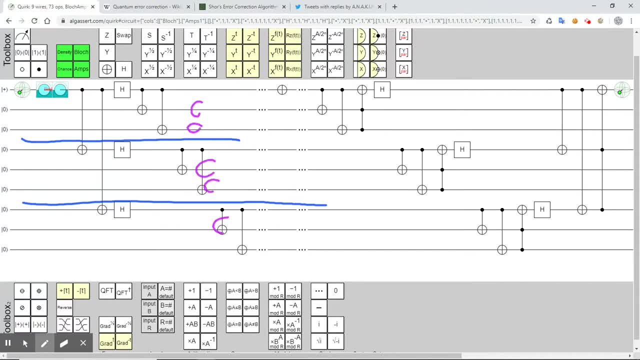 responsible for face corrections, I think. and then the fact that you're doing a control, not in here and in here. so you're basically, you're basically entangling a your state with this register, with this qubit and with this qubit and you know if you. 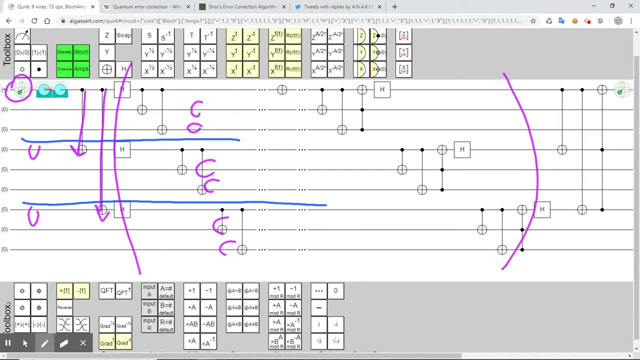 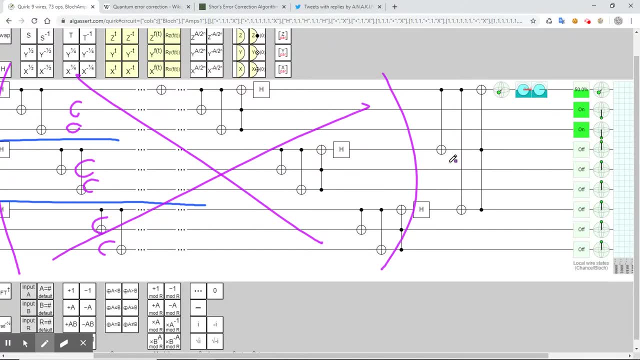 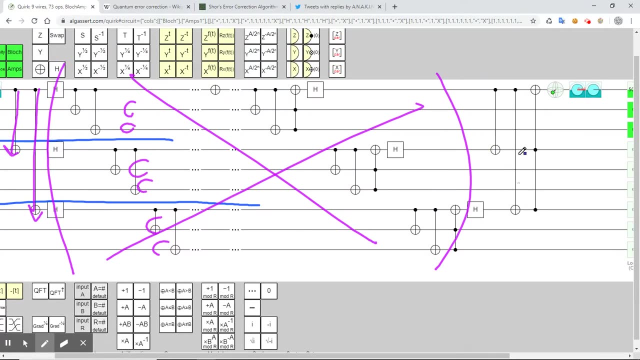 ignore everything that's happening in here, right, let's just let's, let's ignore this for a second. that's really what's. you know what's doing. what this portion of the circuit is doing is saying, okay, so um has anything changing here, right, so let's, let's say: uh, if we, if 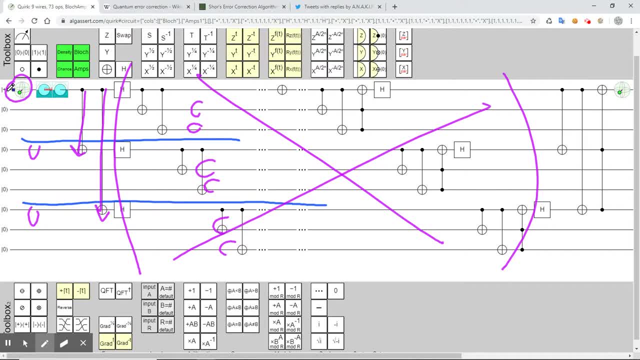 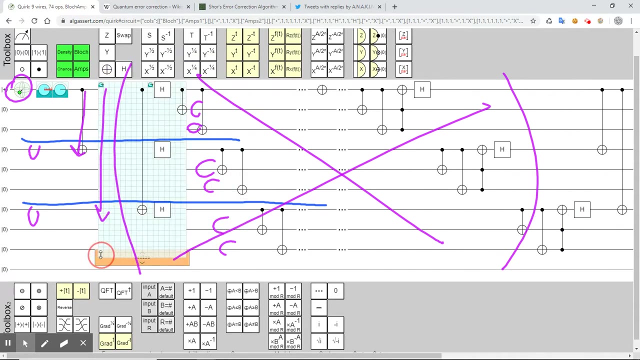 we got a plus stain right. the this is entangled, so we've got a plastic right. this literally means that your amplitudes in here. take a look at the whole system. right, it's the? what's that state? so the all zeros. I'm trying to figure out the. it's complicated to see what. 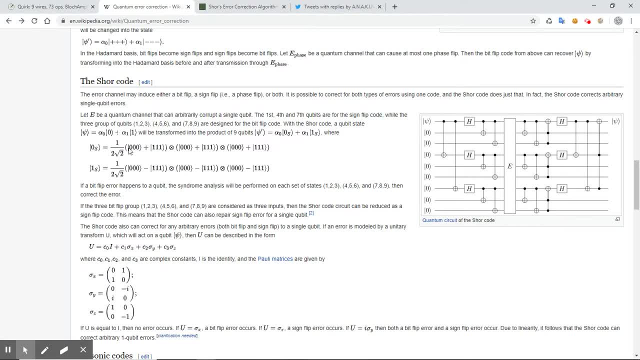 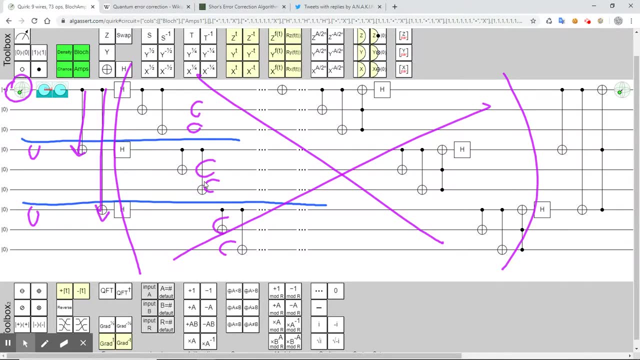 would be the stain. is it the stain, kind of, I think? but essentially, you know, if you, I'm trying to try to reason, reason about this intuitively. if you, let's say, it's a plus state in here, right, and, and so you're, you're entangling it with these and you're. 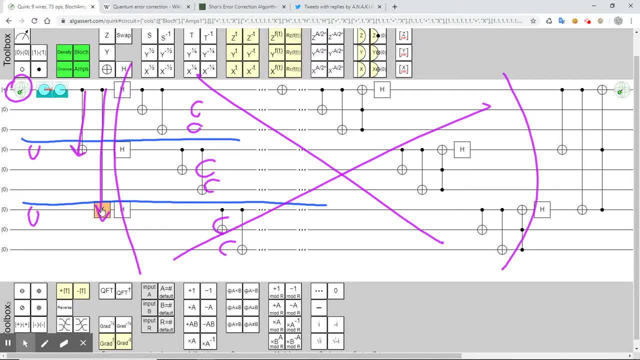 entangling it with this qubit right, and so you're, you're entangling it with this and you're entangling it with this qubit right and, and so you're, you're entangling it with this and you're entangling it with this qubit. 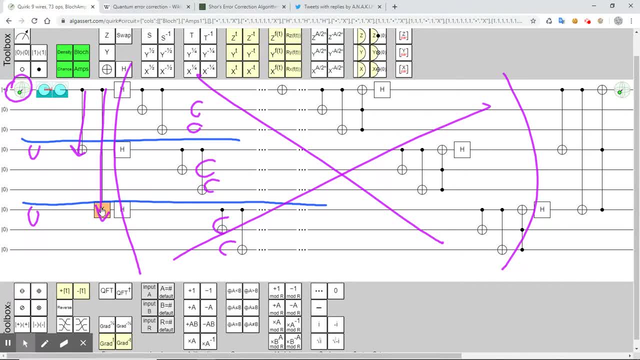 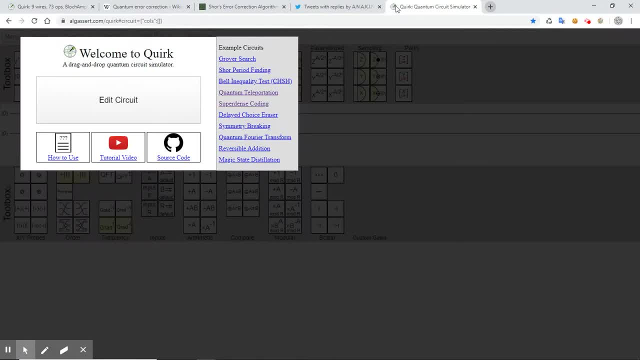 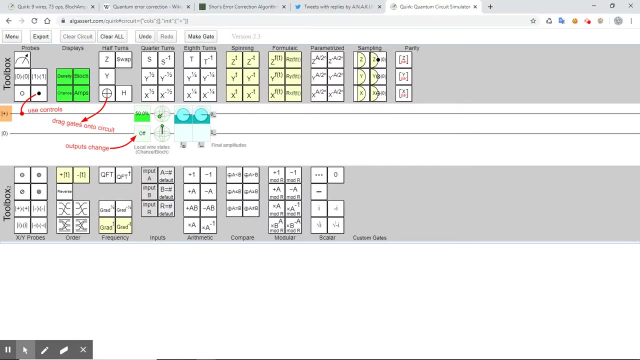 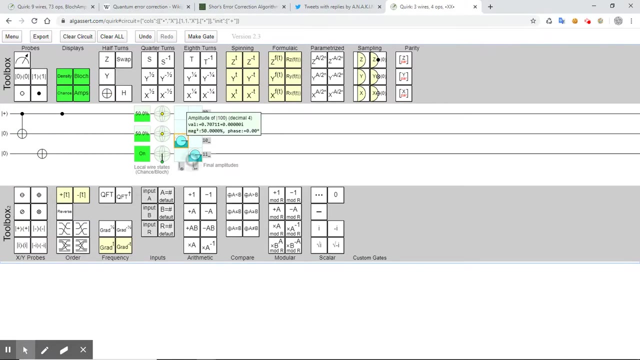 so what have you got as a state in there? you've got is, you've got a um. so if you've got the plus state in here and you do these, you've got the state, this state, sorry, this state. three zeros and three ones exactly. 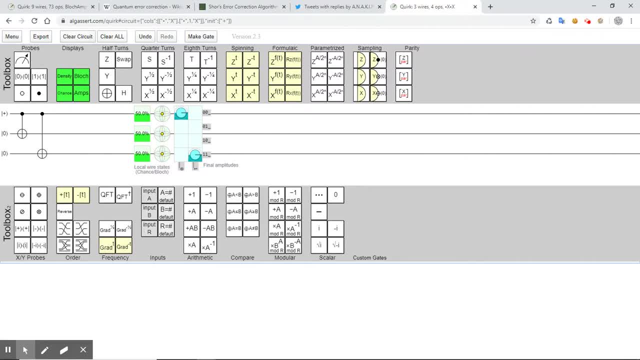 They all agree. And so if something in here in between happens, right, let's say like a bit flip in here, for example, the error correction in here: so what was that? It was a thing like this, like this, and then it was like that. 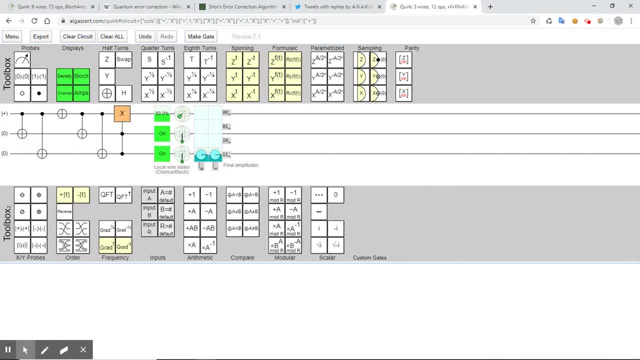 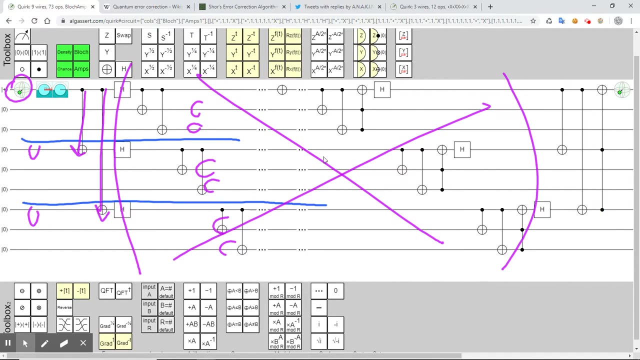 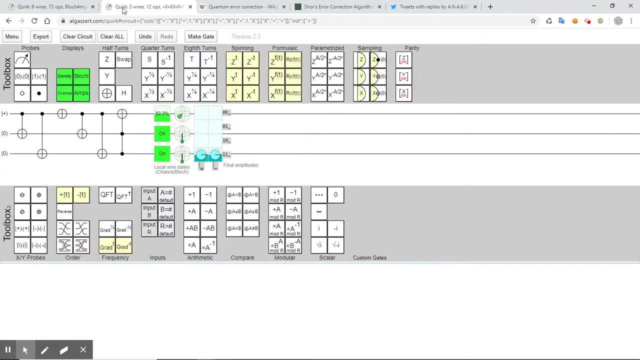 like that and like that, And that's not doing what I expected it to do, I think. Is it this way? No, Yeah, I'm trying to ignore the qubits in between, And this is the error we're simulating. 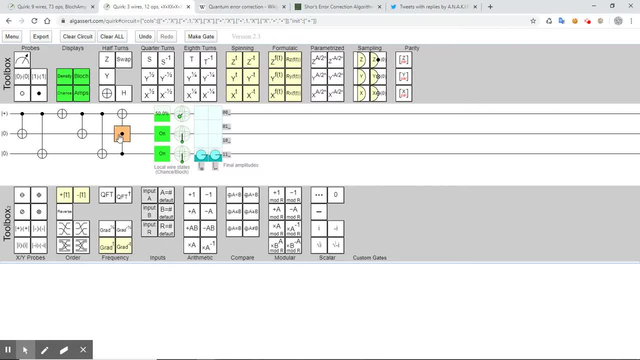 So you're, you're, you want to. you know, what you want to do is you want to make sure that you correct that qubit. So you want to still have a plus in here which you can, which you can. 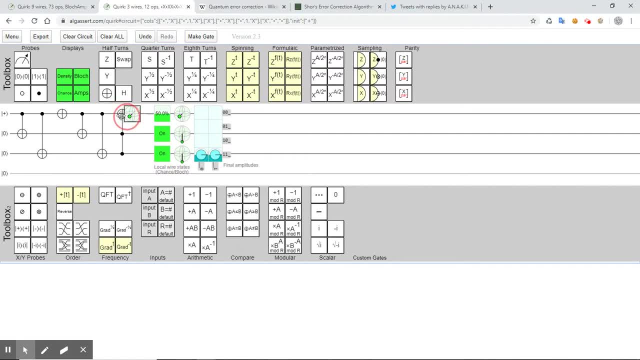 Right, Like you're plus your. what if this is actually protecting you against the? no, that's not the, that's not protecting, that's that. that must be these. I'm trying to think about a way to reason about it. 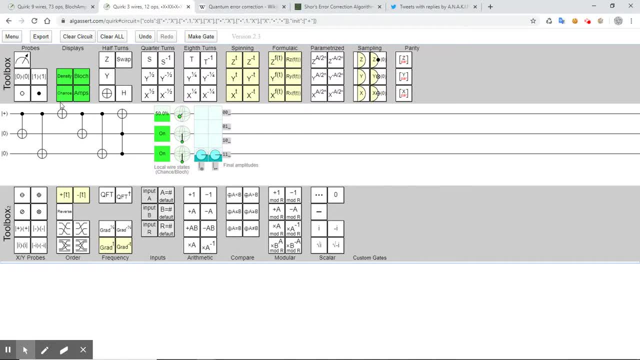 So you entangle these And then, if something like this happens, the still is going to say: you know, for the cases where we've got a 1, I can't reason about this in a smooth way. Give me a second. 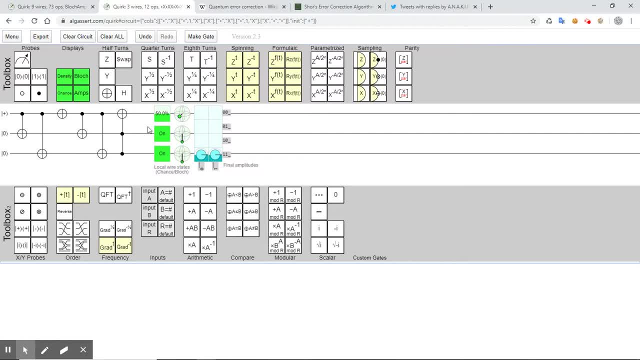 Because essentially it takes that state right, And if it's, maybe that's the wrong way to see it. Like, let's have a simpler state. Let's have like a 1, right? So you've got a 1, and you want to end up with a 1 at the end as well. 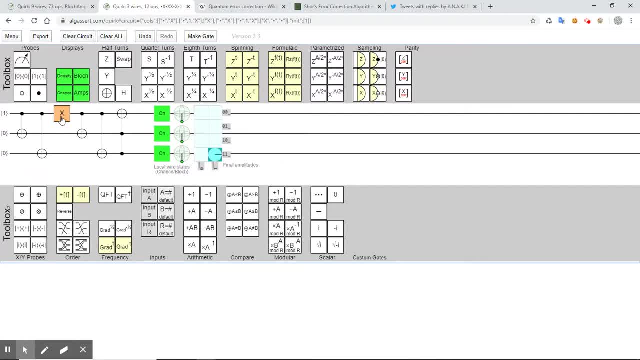 But let's say that now something happens here like a bit flip, right, That's maybe going to be easy. It's going to be easier to see it this way than with a square position state. So this one. what this will do is it will basically flip these two qubits to 1 as well, right? 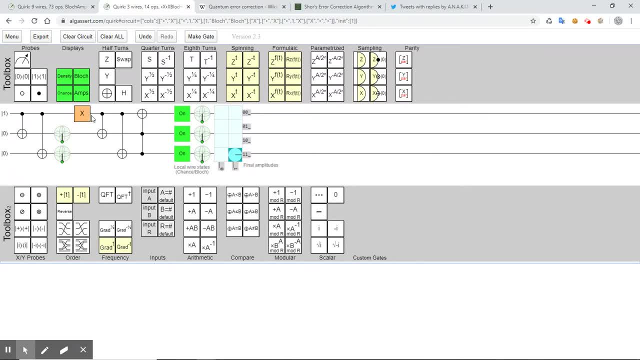 So the and then what's going to happen here is, if there is a- because- let's assume that this gets flipped- then this is going to be now a 0, right, Right. And so this 0 makes these two gates. they don't take place. but then this last one basically self-corrects and puts it back to 1.. 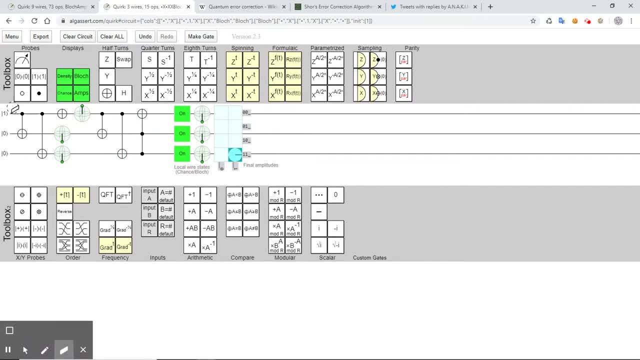 If we were going to do the opposite, say, you know, this is a 0, right And that flips it into a 1. Well then, basically those two things trigger And then again that last TOEFL gate corrects it back again. 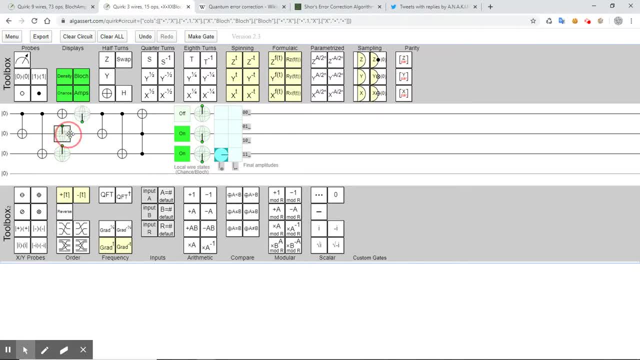 So that's the, yeah, that's the mechanism. Now it works in, it works for all the other states because of the linearity of quantum computing. But I guess that's a lazy explanation of the whole thing, because it's difficult to reason. 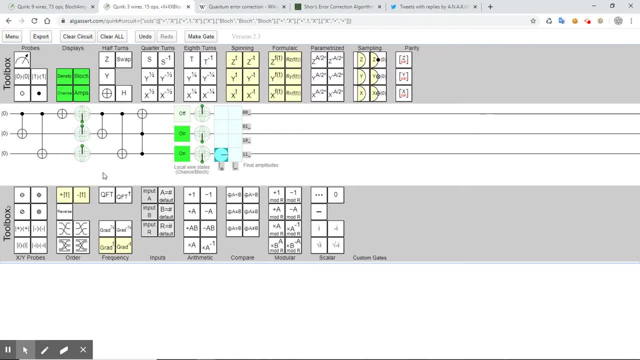 It's really difficult to reason with superpositions in mind, honestly, Because if this is a, let's even say, this is the I state, right, So that's what you've got And that's what you want to get at the end, right? 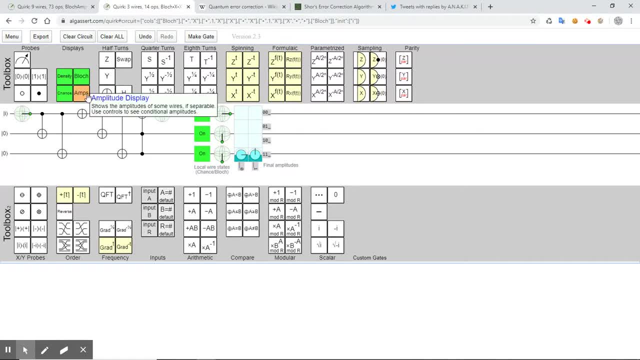 So, if this is the I state right- What you're going to end up with, you need to take a look at the entire system, because now there is, because now there is basically entanglement, So you can't- so you can't easily take a look at this stuff. 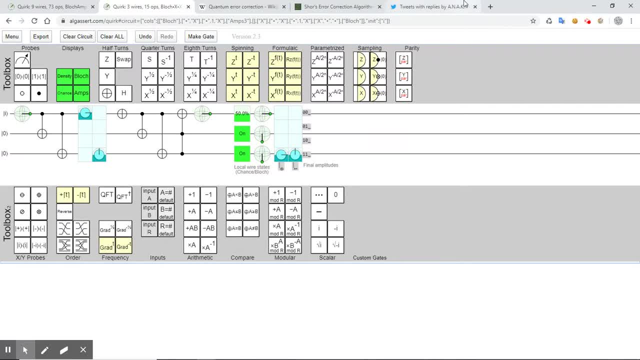 That's you just turning to be a bit longer than it is. So you can't just take a look at this stuff. That's you just turning to be a bit longer than it is. So you can't just take a look at this stuff. That's you just turning to be a bit longer than it is. 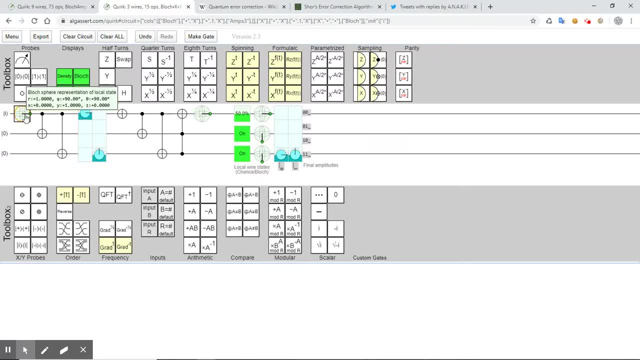 So I think I'll have to finish it in a second, But basically that's that's what it does. So so, so what this what this is doing if you take a look at the amplitudes here before it's moving that. 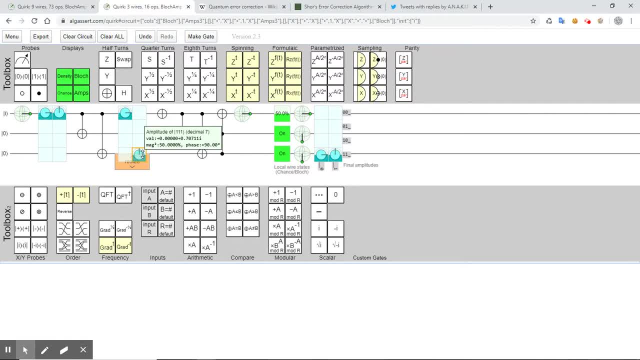 that one all the way here to the one one one. So it's encoding, this is kind of attaching the zero and the zero and the one component and the two ends of your superposition. So if, if it now a bit flip happens, 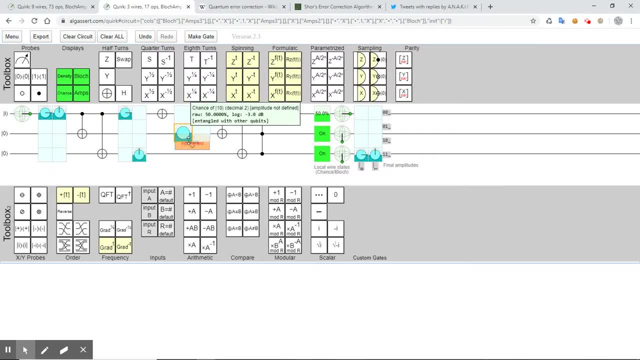 which would basically mean that the things get like you know. mirrored you, you would still have. so what you still have now is the. so how does this so that that self correction happens in a similar fashion? because you're okay, Let's. let's put it this way: 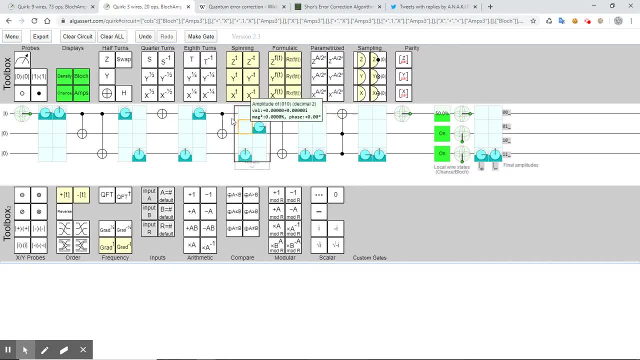 Yeah, It's, it's doing these, it's really it's doing this. so if nothing happens, let's say nothing happens. he is where there happens. nothing happens, then these things. they just kind of reversed that thing And go back to that state. 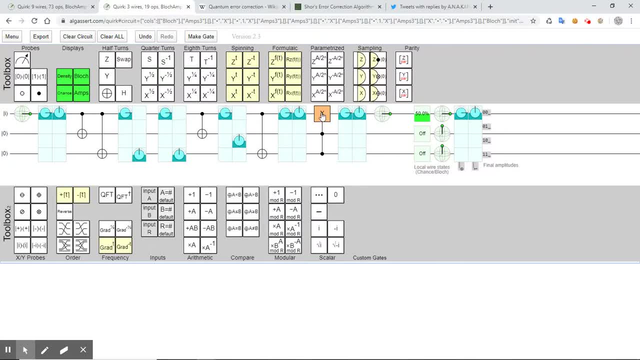 Basically because that gate doesn't have an influence. So this is an computing that maybe will be easier to seem. that took, yeah, it's, it's basically uncomputing, but if in detail we we come back again. 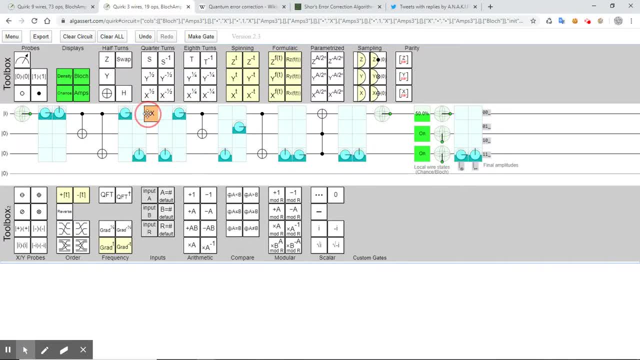 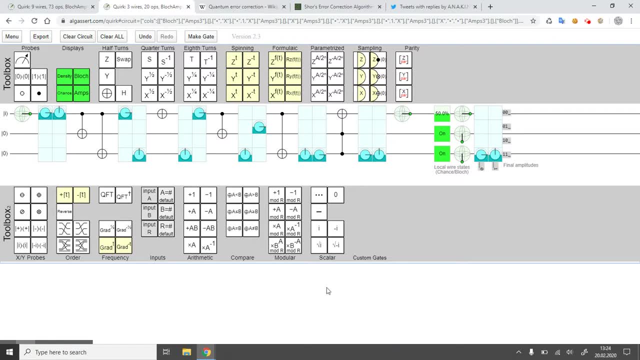 something happens, right, then you're, then you're gonna have that effect that this uncomputation it's gonna end up it's gonna tap down here just at the end of the day. but I still understand why this is why this then in here and not in here. 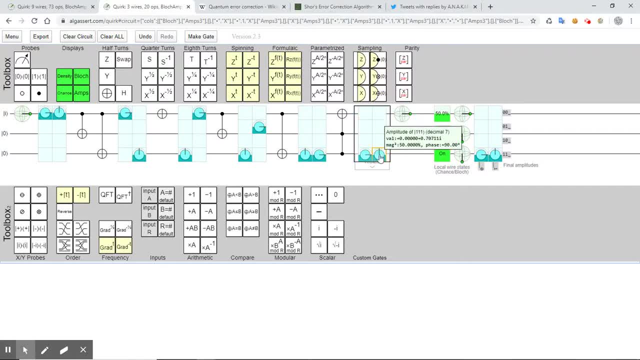 but still it's giving us the right blocks here. that's what I don't fully understand. but this is because the stricter reason with with states in superposition. but okay, I'll turn that into, I guess, like probably a couple more videos, but intuitively I think that's what's. that's what's happening, this. 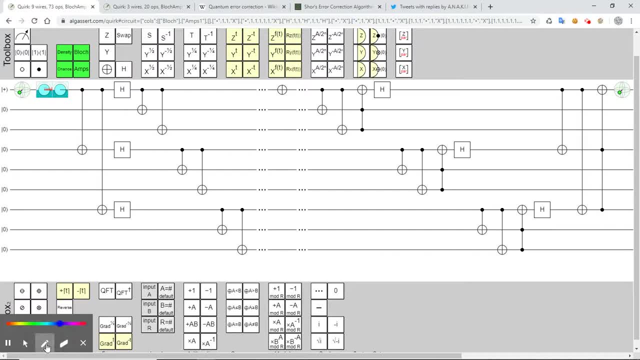 portion. let me clean that up. so this portion here and here takes care of the fifth flip and these other ones in here they care of the face flips. so we'll take a look at the face flips in the next video, probably, and then we'll just try to put everything together. but I just want to.